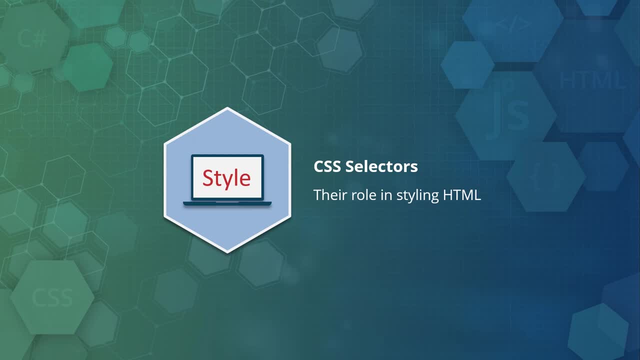 and values and things like that we put alongside the name of the HTML tag itself. So, for example, we can attach a class to a particular element, We can attach an ID, a name. These are all selectors, But what I want to focus on in this video are those attribute, equal values, those attributes. 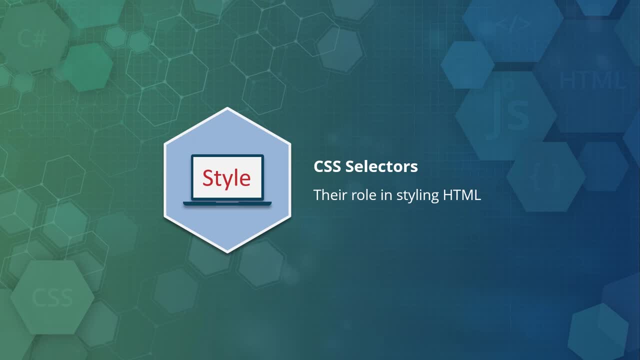 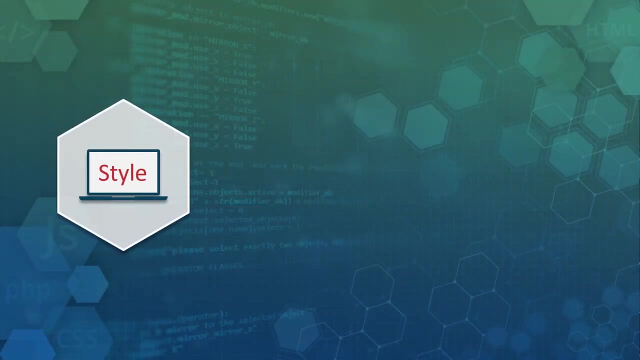 that we add to HTML elements. Those are not so common, but they provide excellent value when it comes to selecting things on a web page. So whenever we have an element and we have some kind of an attribute attached to that element, we can or just simply looking. 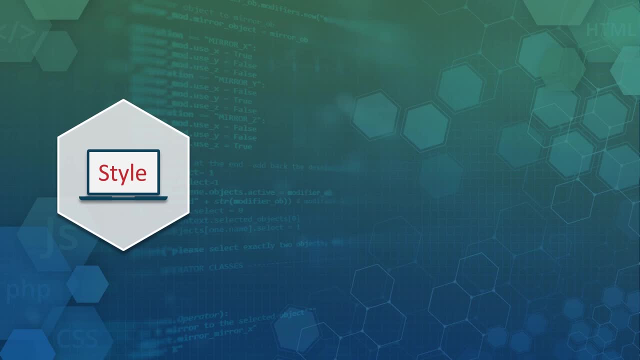 at the attribute, we can see that the attribute is already a selector in itself. So, for example, we might be searching for all of the classes that exist on the page And if there is a class, then we can apply a particular style to it, or we can search for IDs, etc. Then 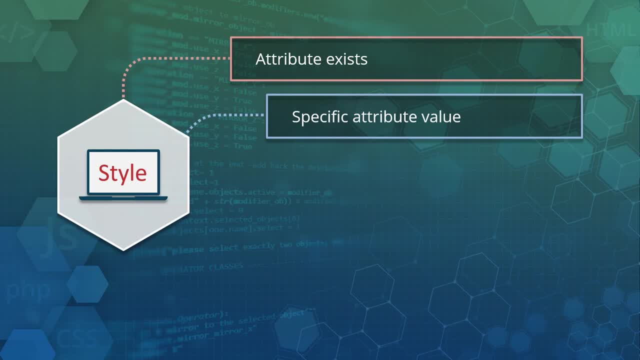 we can search specific value that that attribute has. So, for example, the attribute is on the left, the value is on the right and we can search for all of those elements that have that specific value. We can even search with a wildcard value. So, for example, if 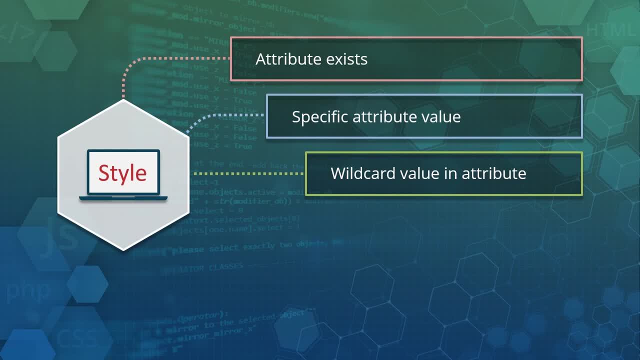 the attribute exists on the page and it contains a few letters. let's say, then we can search for anything with the value that has those letters in it. Now the wildcard value is very similar to searching for a specific value inside of a list. So, for example, we may: 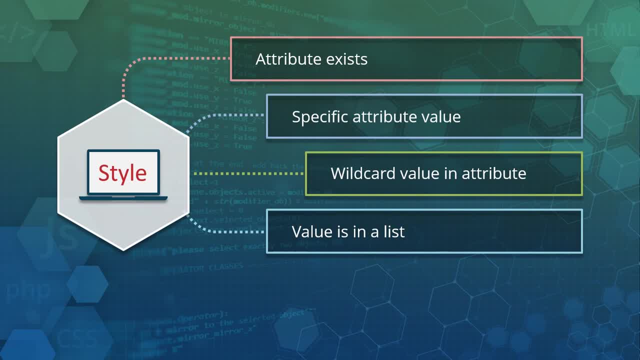 have a particular pattern of letters that we're looking for and we're simply searching to see if that exists. So value in a list and wildcard value are very similar. We can also search for a particular pattern that starts the value part of the attribute. 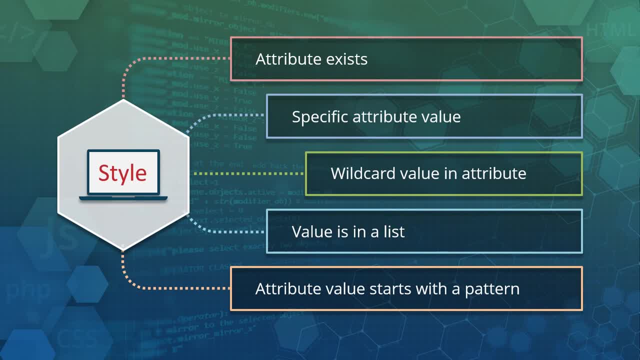 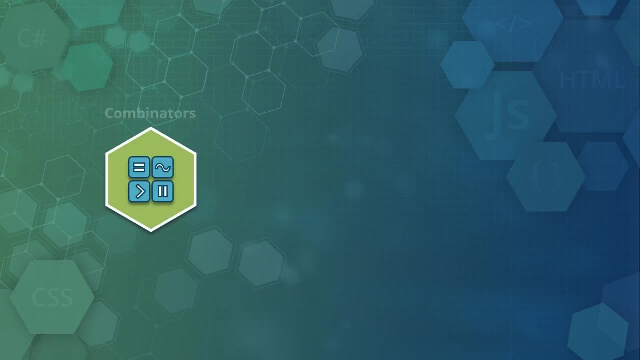 So, for example, if it starts with the letter VAL, then we know that we want to select those particular elements, And there are a couple more like these, but these are the more important ones. There are some newer types of selectors, So, for example, combinators, Combinators,